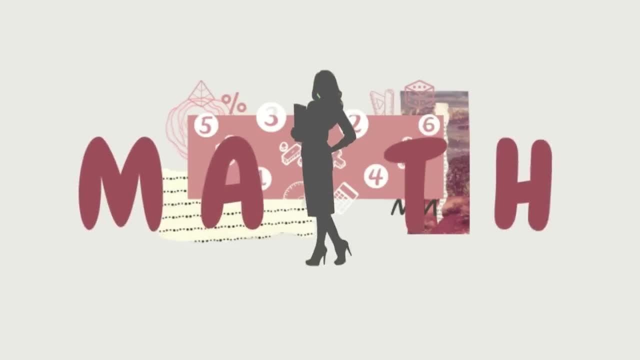 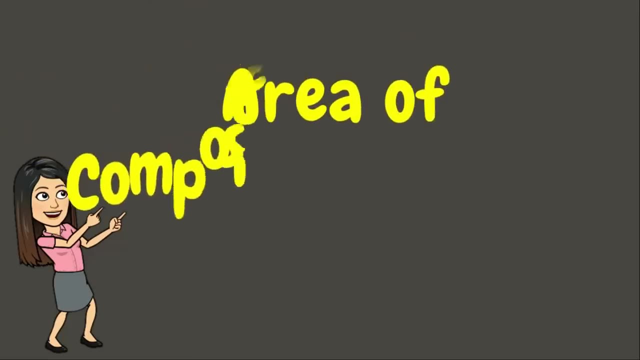 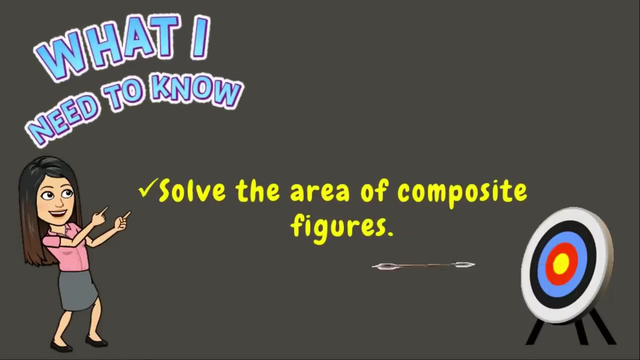 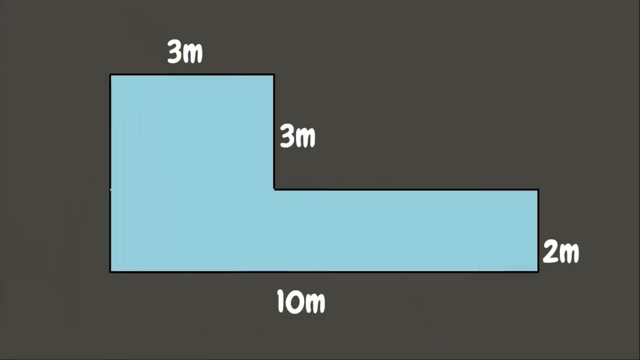 Hello, dear students, welcome back to my classroom For today's lesson. you are going to learn how to solve the area of composite figures. Let us begin. Let's take a look at our first example. Let's find out the area of this composite figure. But wait, do you know what? 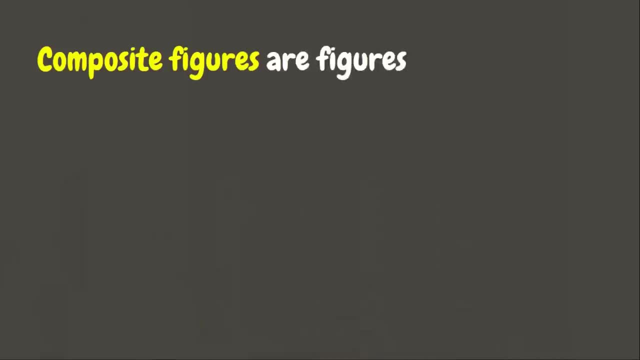 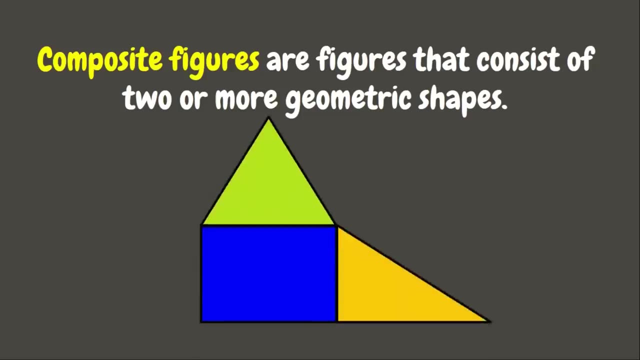 composite figure means. A composite figure is a figure that consists of two or more geometric shapes. For example, we have here a composite figure which consists of three geometric shapes. It has two triangles and one square. To find out the area of this composite figure, we just simply need to get the area of each. 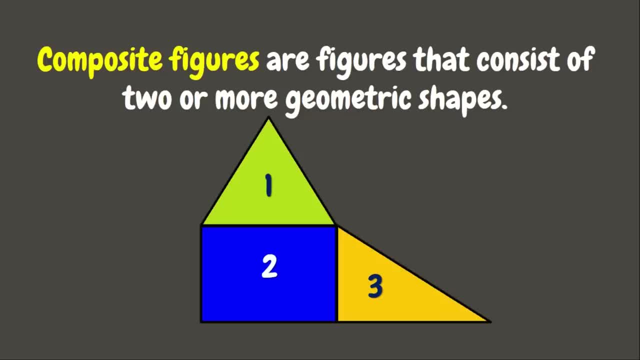 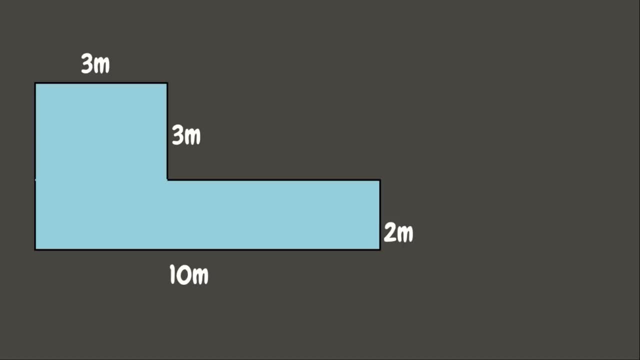 geometric shape and combine them together. Now let's try and go back to our example. The first thing that we need to do to get the area of this composite figure is to divide or separate this into basic shapes. Here we can see that we can divide this into two basic 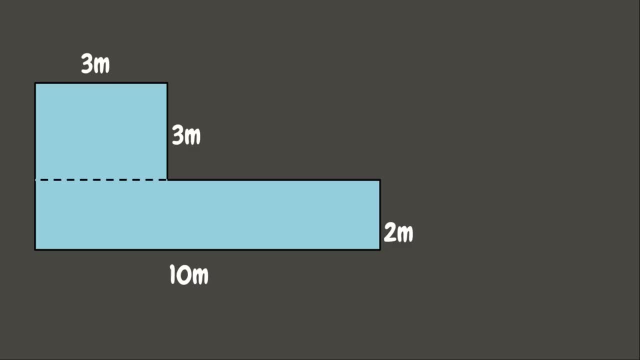 shapes, which are the rectangle and the square. Now that we have separated them, the next thing that you need to do is to get the area of each shape. Let's try to get the area first of the square. Again, the formula for the 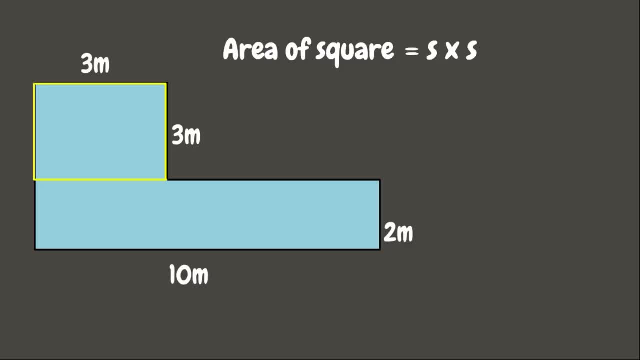 area of the square is side times side. Here, the measure of each side is 3 meters. Now let us multiply 3 meters times 3 meters is 9 square meters. Therefore, this is the area of the square. Next thing that we need to do is to get the area of the rectangle, The formula for the area of the. 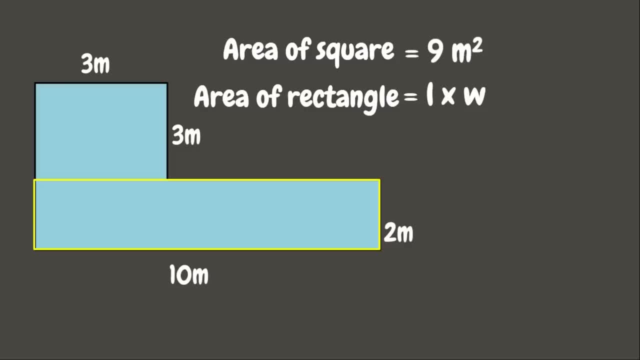 rectangle is length times width. Here the measurement of the length is 10 meters, while the width is 2 meters. Now let us multiply 10 meters times 2 meters is Great job. It is 20 square meters. Therefore, this is the area of the rectangle. 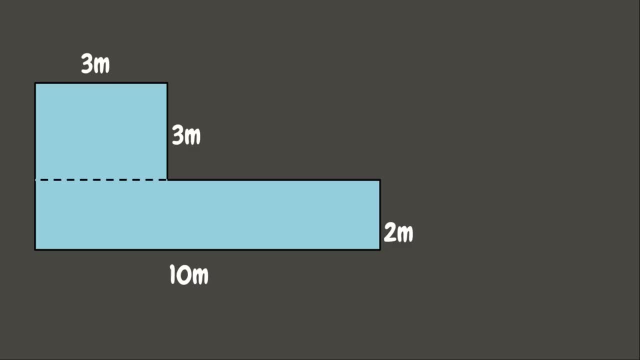 shapes, which are the rectangle and the square. Now that we have separated them, the next thing that you need to do is to get the area of each shape. Let's try to get the area first of the square. Again, the formula for the 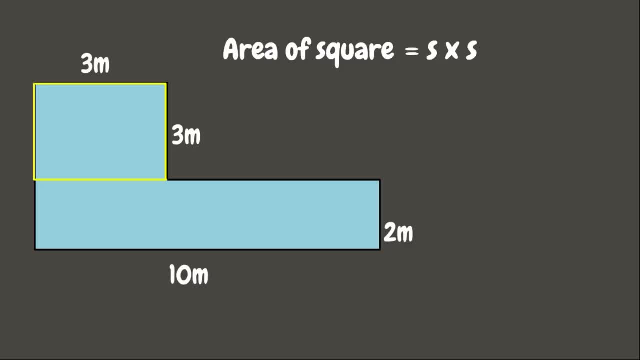 area of the square is side times side. Here, the measure of each side is 3 meters. Now let us multiply 3 meters times 3 meters is 9 square meters. Therefore, this is the area of the square. Next thing that we need to do is to get the area of the rectangle, The formula for the area of the. 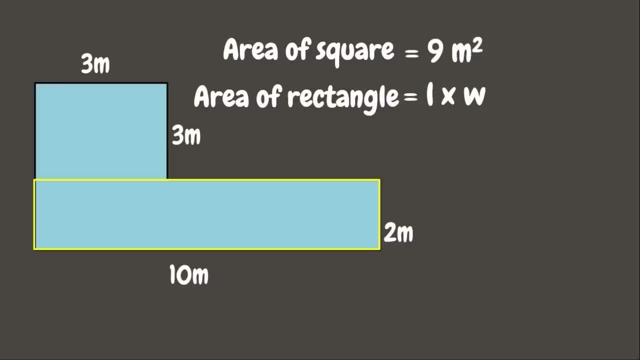 rectangle is length times width. Here the measurement of the length is 10 meters, while the width is 2 meters. Now let us multiply 10 meters times 2 meters is Great job. It is 20 square meters. Therefore, this is the area of the rectangle. 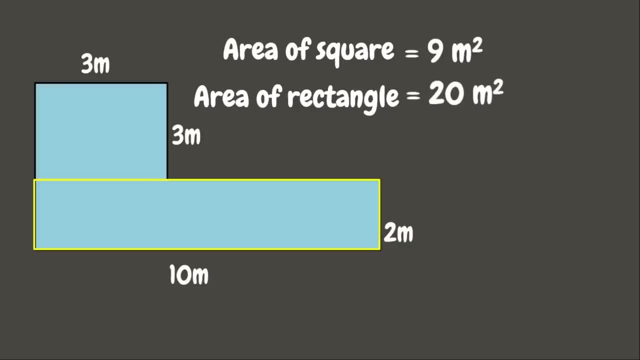 Now the next thing that we need to do is to combine the two areas together. This means that we need to add 9 square meters and 20 square meters, And that would be 29 square meters. Now, this is the area of this composite figure. Wonderful, Now let's go and have a 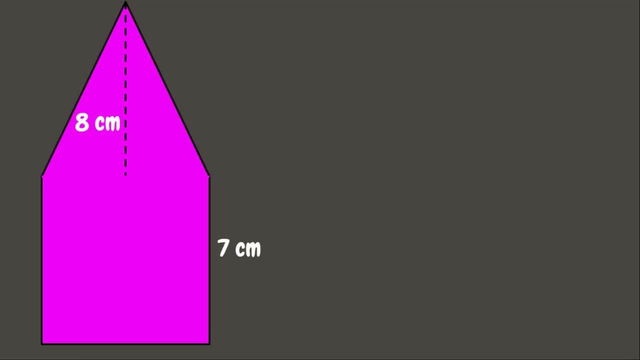 look of another example. This time we have another composite figure. Again, the first thing that you need to do is to divide or separate this into basic shapes. Here we can divide this composite figure into two basic shapes, Which are the triangle and the. 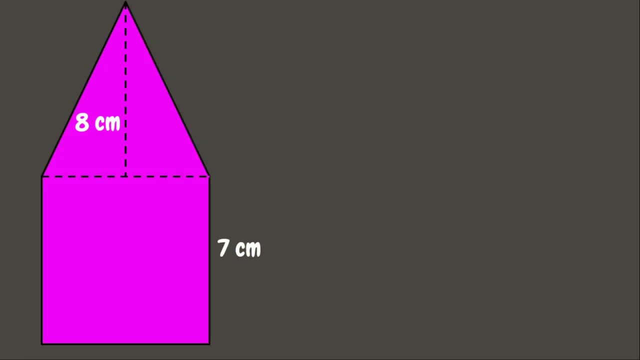 square. The next thing that we need to do is to get the area of each shape. Let's first get the area of the square And then divide the area of the rectangle into 2 basic shapes. So we have one triangle, one square and one circle. Now we have a triangle, So when we 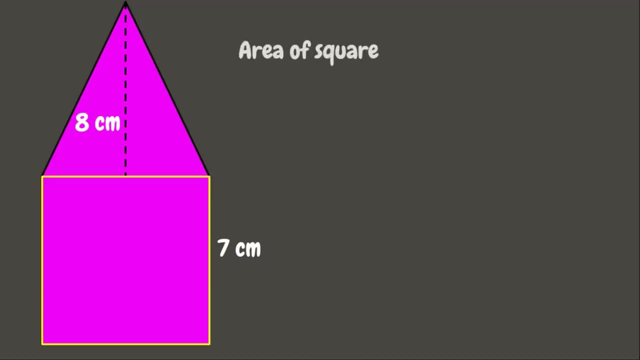 square. again, the formula for the area of the square is side times side. here the side of the square measures seven centimeter. this means that we are going to multiply seven centimeters by seven centimeters and that would be 49 square centimeters, and that is the area of the square. now let's go. 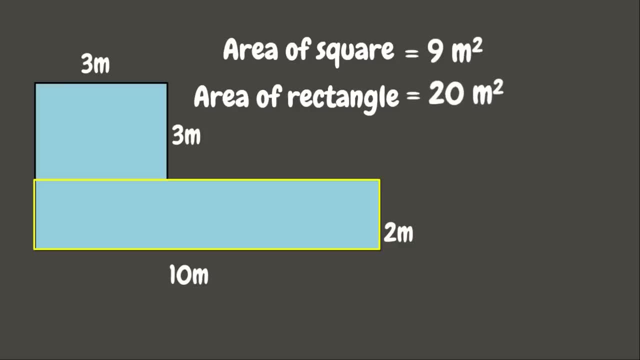 Now the next thing that we need to do is to combine the two areas together. This means that we need to add 9 square meters and 20 square meters, And that would be 29 square meters. Now, this is the area of this composite figure. Wonderful, Now let's go and have a 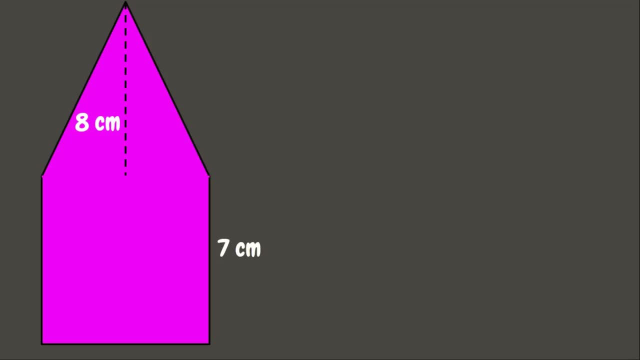 look at another example. This time we have another composite figure. Again, the first thing that you need to do is to divide or separate this into basic shapes. Here we can divide this composite figure into two basic shapes, which are the triangle and the square. The next thing that we need to do is to get the area of each shape. 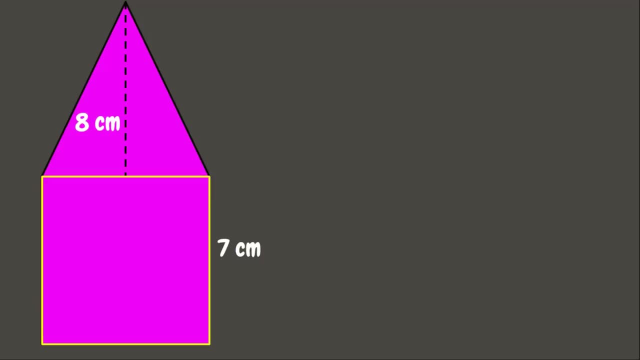 Let's first get the area of the square. Let's get point of the rectangle, Clapping class ichtet area of each shape. find the area of each shape. Let's first get the area of the square. again. the formula for the area of the square is side times, side, here the side of the. 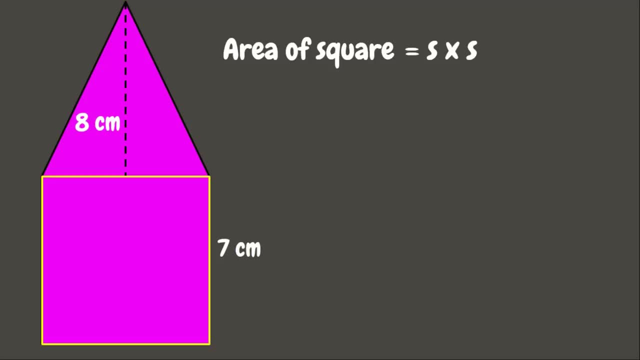 square measures seven centimeter. this means that we are going to multiply seven centimeters by seven centimeters and that would be 49 square centimeters, and that is the area of the square. now let's go and get the area of the triangle. the formula for the area of the triangle is: base times height. 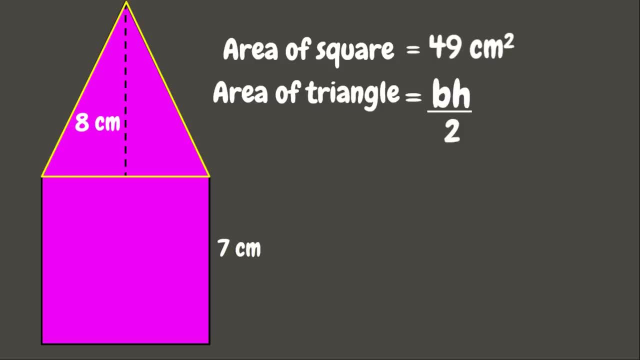 divided by two. here we can say that the measurement of the base is seven centimeters, since the size of the square are equal. now let us multiply. we have the base seven centimeter times the height, which is eight centimeter, divided by two. seven centimeters times eight centimeters is: 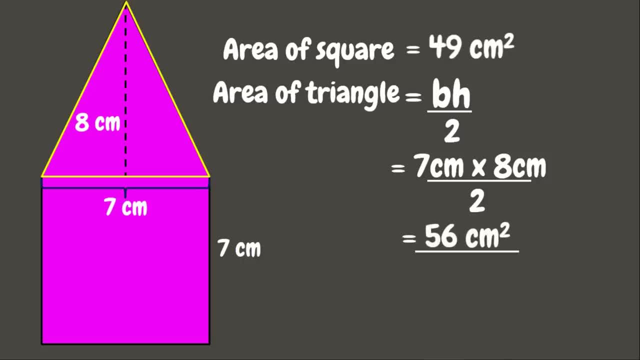 56 square centimeters. now let's divide it into two, and that would be 28 square centimeters, and that is the area of the triangle. now, next thing that we need to do is to combine the two areas. now let us add: 49 plus 28 is wonderful. it is 77 square centimeters. therefore, this is: 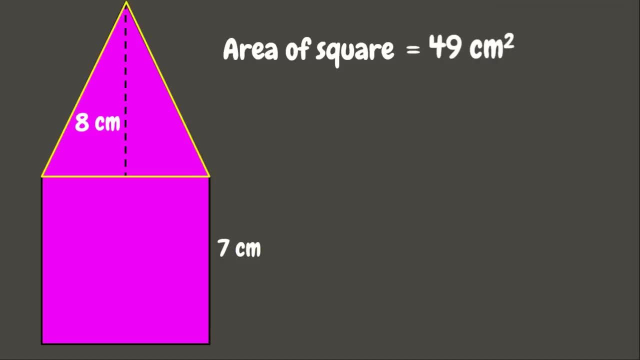 and get the area of the triangle. the formula for the area of the triangle is base times height divided by two. here we can say that the measurement of the base is seven centimeters, since the size of the square are equal. now let us multiply. we have the base seven centimeter times the height. 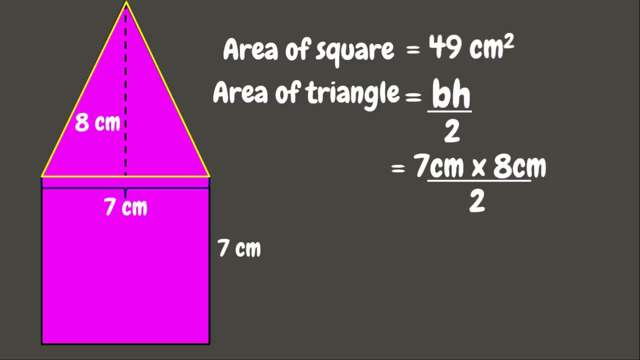 which is eight centimeter, divided by two, seven centimeters times eight centimeters is 56 square centimeters. now let's divide it into two, and that would be 28 square centimeters, and that is the area of the triangle. now, next thing that we need to do is to combine the two areas. 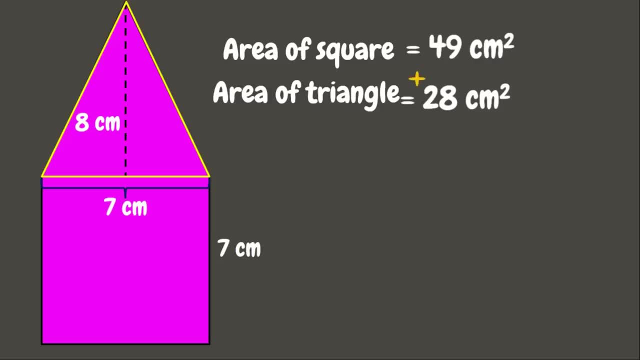 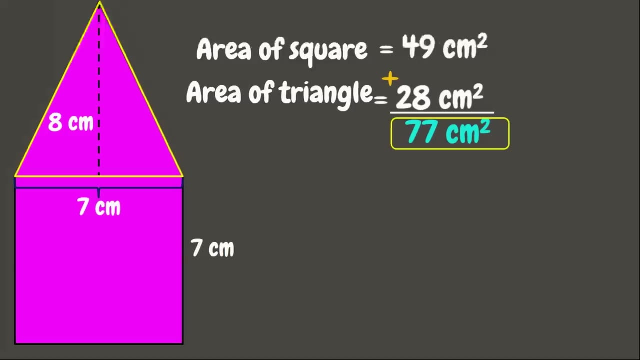 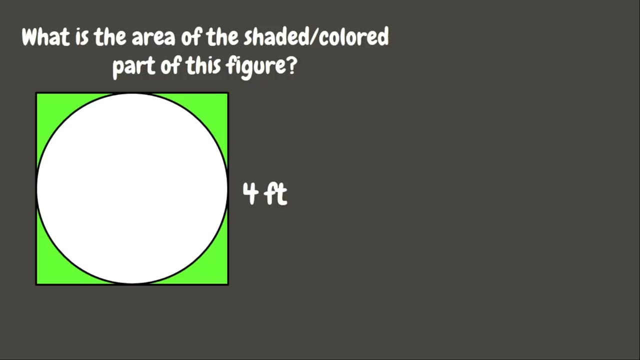 now let us add: 49 plus 28 is wonderful. it is 77 square centimeters. therefore, this is of this composite figure. awesome job. now let's move on and have another example. this time we need to get the area of the shaded, or the colored part of this. 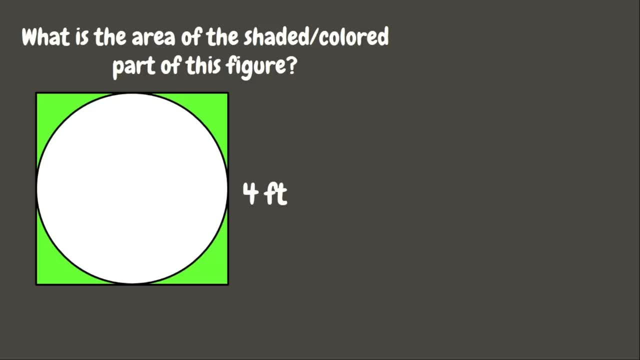 figure. as we can see, this figure is already separated into two shapes. we have the circle in the square and let us get first the area of the square. let us multiply side by the side, so that would be 4 times 4 and that is 16 square. 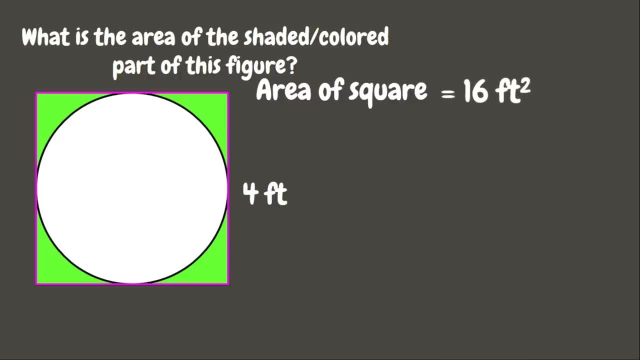 feet. next let's get the area of the circle. the formula for the area of the circle is PI R squared, where the value of the PI that we are going to use is 3.14. next we have the radius. here we can say that the diameter of this circle is 4 feet and the radius 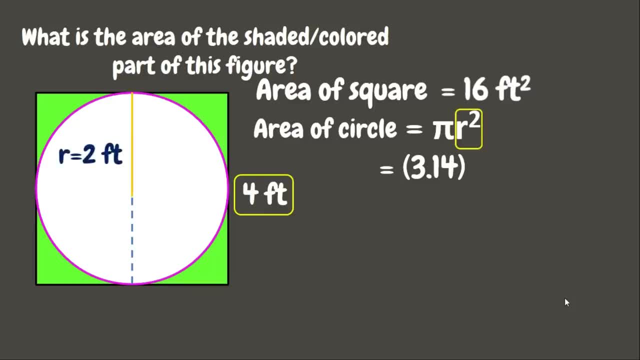 which is half of the diameter, would be 2 feet. therefore, we need to multiply 2 feet 2 times 2 itself, so that would be 2 feet times 2 feet, 2 feet times 2 feet. Now let us solve: We have 3.14 times 4 square feet. 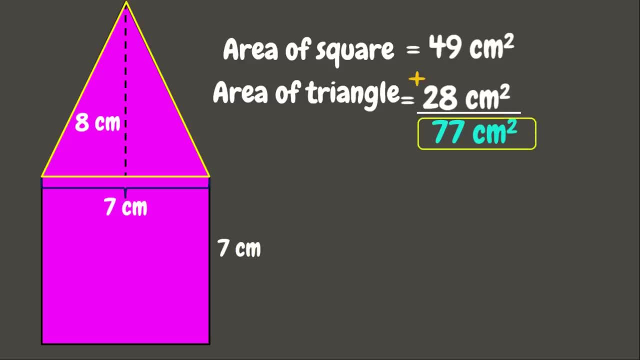 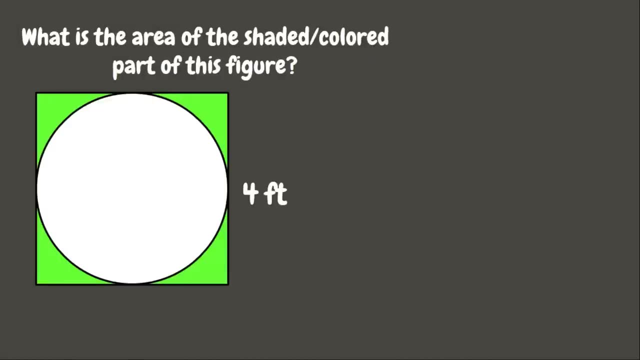 C of this composite figure. awesome job. now let's move on and have another example. this time we need to get the area of the shaded or the colored part of this figure. as we can see, this figure is already separated into two shapes. we have the circle in the square, and let us get first the area of the square. let 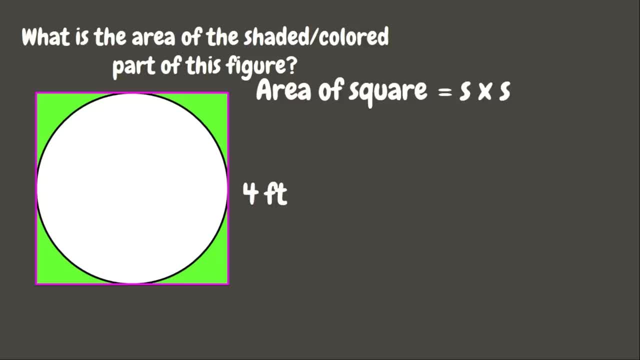 us multiply side by the side, so that would be 4 feet times 4 feet and that is 16 square feet. next let's get the area of the circle. the formula for the area of the circle is PI R squared, where the value of the PI that we are. 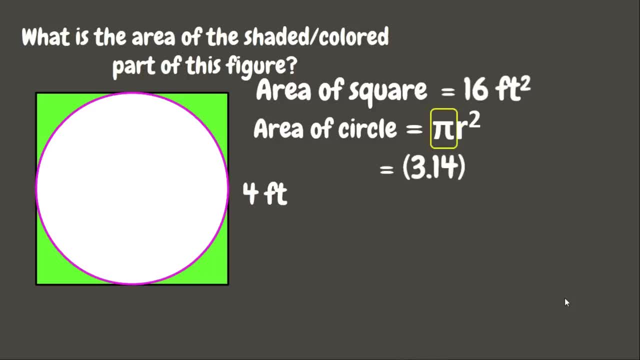 going to use is 3.14. next we have the radius. here we can say that the diameter of this circle is 4 feet and the radius which is half of the diameter would be 2 feet. therefore, we need to multiply 2 feet 2 times 2 itself. so that would be. 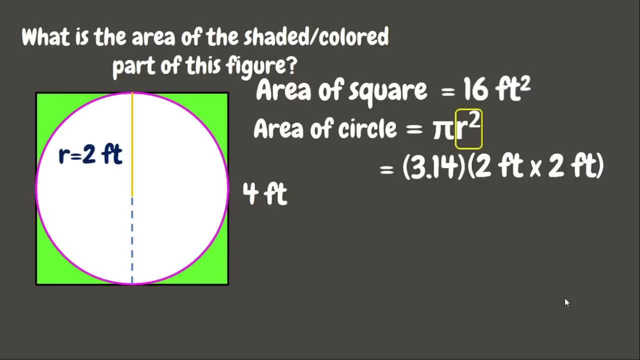 2 feet, 2 feet. Now let us solve. We have 3.14 x 4 square feet And that is 12.56 square feet, And this is the area of the circle. Now, in the given question, We need to find out the area of the shaded or the colored part of this figure. 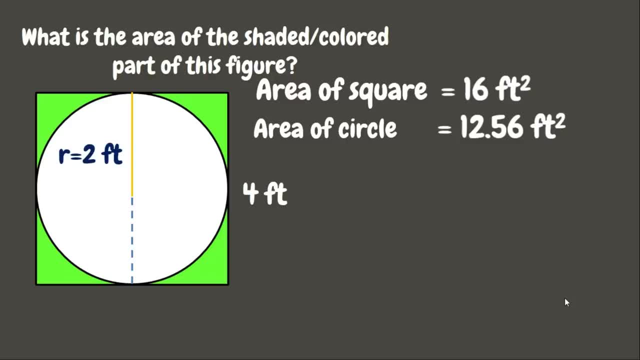 Here, the colored part is the green part. This means that we only need to get the area of the green part. Therefore, instead of adding the areas together, We are going to subtract Now. let us subtract 16 and 12.56, And that would be 3.44 square feet. 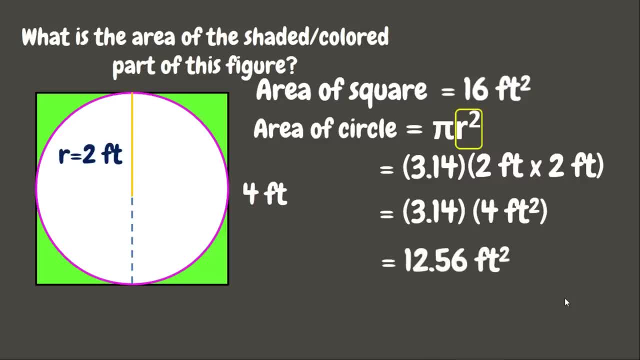 And that is 12.56 square feet And this is the area of the circle. Now in the given question, We need to find out the area of the shaded or the colored part of this figure. Here the colored part is the green part. This means that we only need to get the area of the green part. 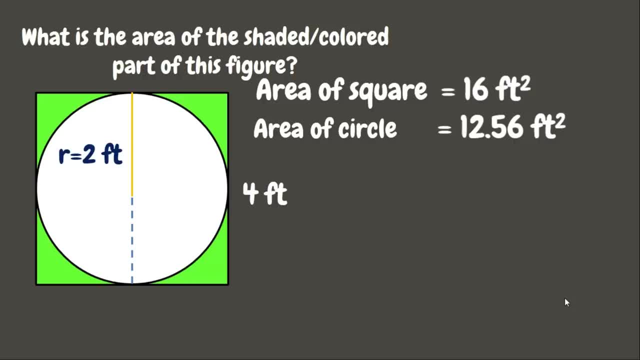 Therefore, instead of adding the areas together, We are going to subtract. Now. let us subtract 16 and 12.56, And that would be 3.44 square feet. Therefore, this is the area of the colored, or the shaded part of this figure. Wonderful. 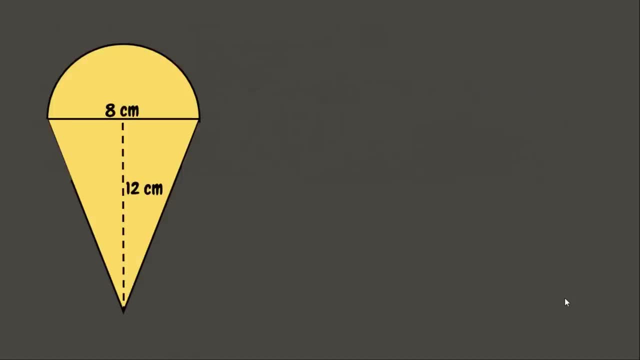 Now let us move on to our last example. Here we can see that the figure is already divided into basic shapes. We have the semicircle and the triangle. First let us get the area of the triangle Again. the formula for the area of the triangle is: 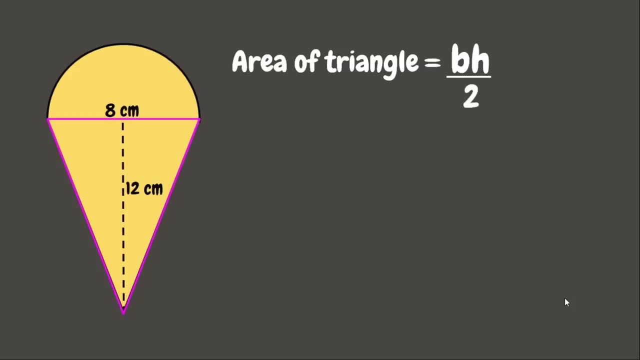 Base times height divided by 2. Here the base is 8 centimeters, While the height is 12 centimeters. So that would be 8 centimeters times 12 centimeters divided by 2. 8 centimeters times 12 centimeters is 96 square centimeters. 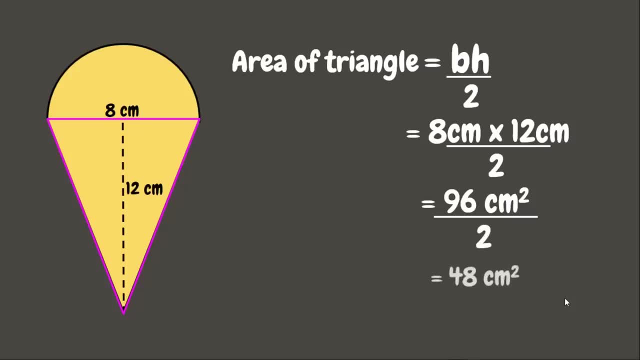 And let us divide it by 2, And that would be 48 square centimeters. This means that this is the area of the triangle. Next, let us find out the area of the semicircle. The formula for the area of the semicircle is: 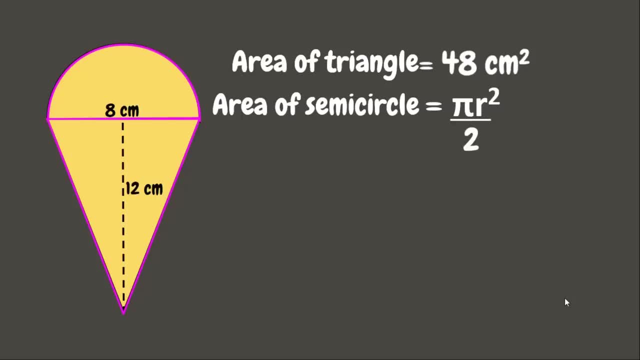 Pi r squared, divided by 2. Again, the value of the pi that we are going to use is 3.40. Next, we are going to multiply that to the square of the radius. To get the radius, we need to divide the diameter into 2. 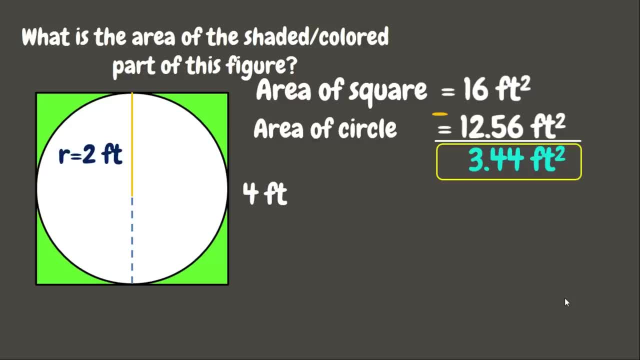 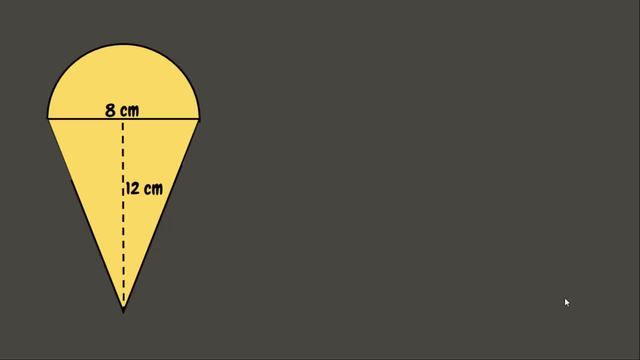 Therefore, this is the area of the colored, or the shaded part of this figure. Wonderful. Now let us move on to our last example. Here we can see that the figure is already divided into basic shapes. We have the semicircle and the triangle. First let us get the area of the triangle. 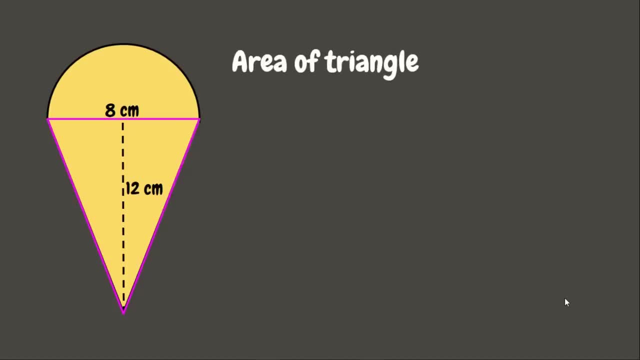 Again, the formula for the area of the triangle is Base times height divided by 2. Here the base is 8 cm, While the height is 12 cm. So that would be 8 cm times 12 cm divided by 2. 8 cm times 12 cm is 96 square cm. 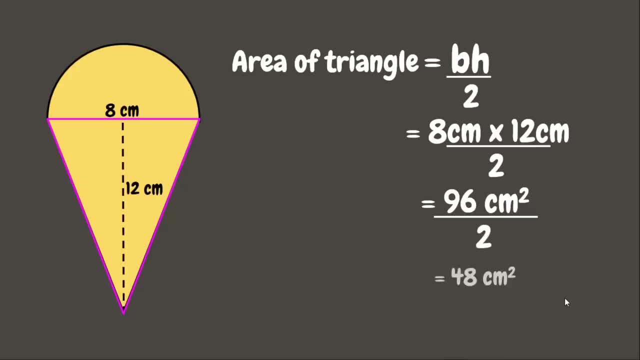 And let us divide it by 2, And that would be 48 square cm. This means that this is the area of the triangle. Next, let us find out the area of the semicircle. The formula for the area of the semicircle is Pi r squared divided by 2. 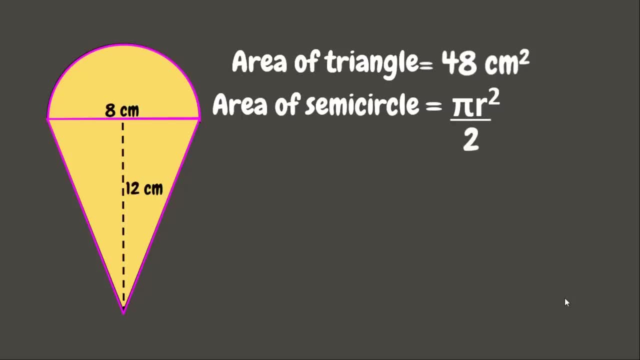 Again, the value of the pi that we are going to use is 3.40. Next, we are going to multiply that to the square of the radius. To get the radius, we need to divide the diameter into 2. The diameter measures 8 cm. 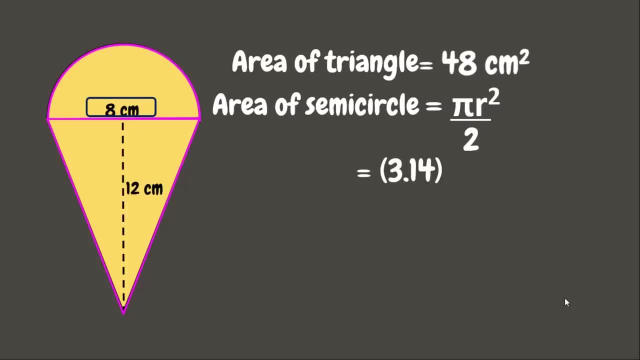 So if we divide that into 2, That would be 4.4 cm. That would be 4.4 cm. So that is our radius. Now that would be 4 cm times 4 cm. Now let us solve. We have 50.24 square cm divided by 2. 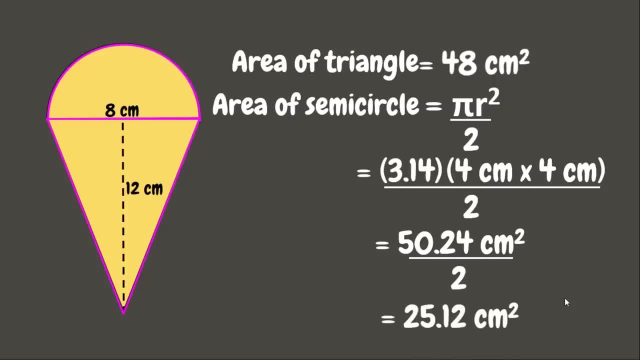 And the answer would be 25.12 square cm, And that is the area of our semicircle. Now the next step that we need to do is to find the area of the semicircle, And the next step that we need to do is to combine the 2 areas together. 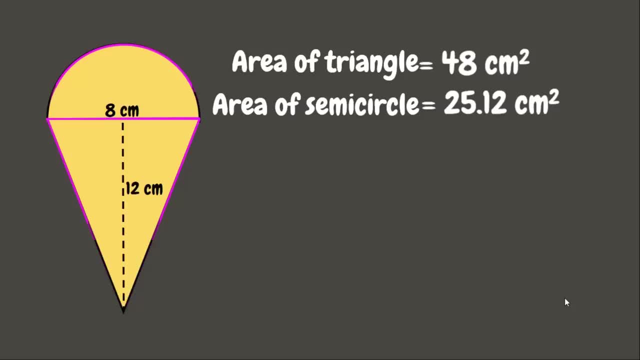 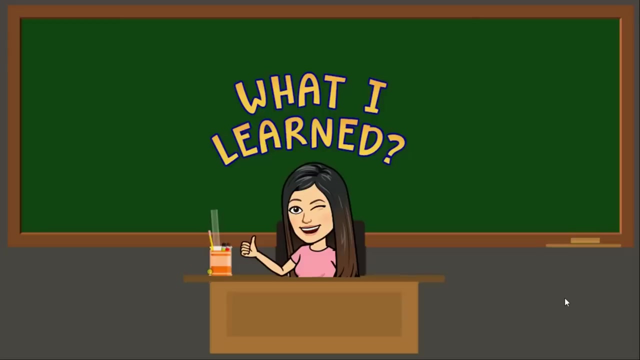 And that is the area of our semicircle, And the area would be 73.12 cm squared. Now, this is the area of this composite figure. Wonderful, You made it this far, students. Now here are the things that you learned today. You made it this far, students.